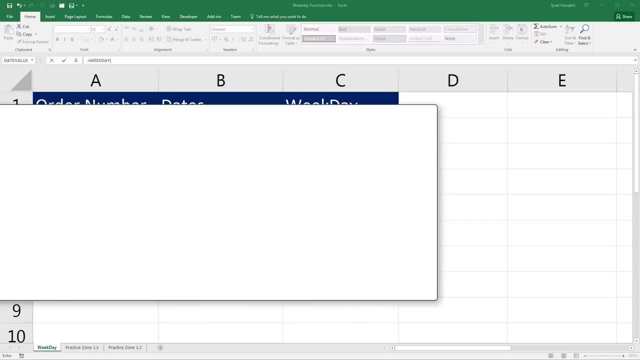 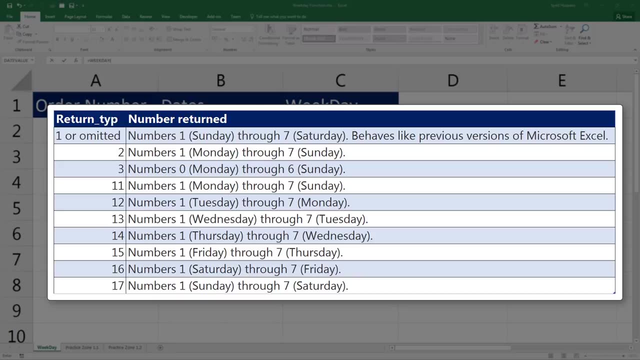 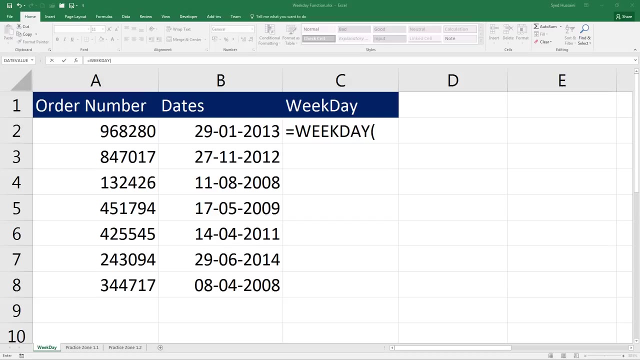 1,, 2, 7.. You can pause the video here and take a look at the table on the screen to see the numbers that are provided. That will help you to decide on the return type values. You can also use the link in the video description to go to Microsoft website. that will help you to learn more about return types. 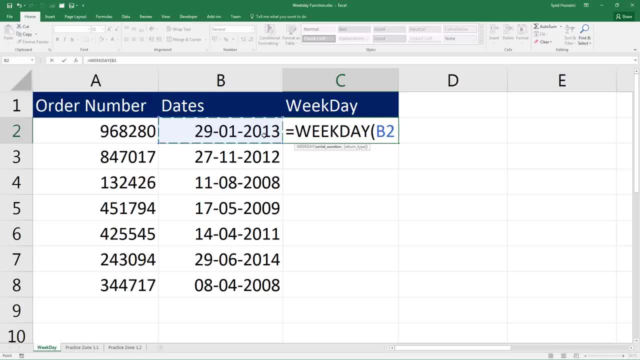 Let us go ahead and select B2 and without giving any return type, I will simply close the bracket and press enter on my keyboard. Now this one will return me the number for that date. So that's the third day of the weekday. The third day of the weekday is that week. So if I am starting from Sunday, Monday, Tuesday, that's the day. If I drag this down, I will have more weekdays generated. 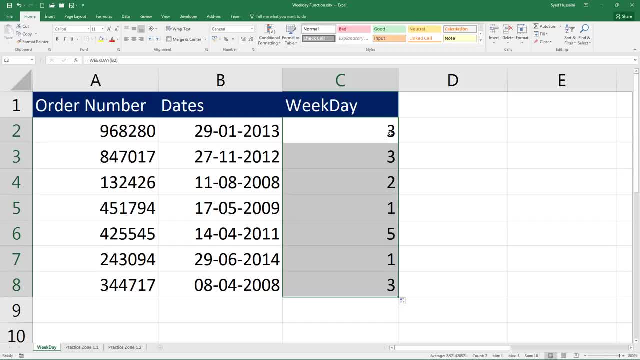 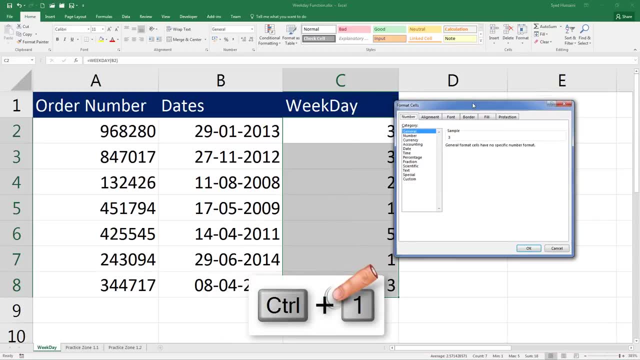 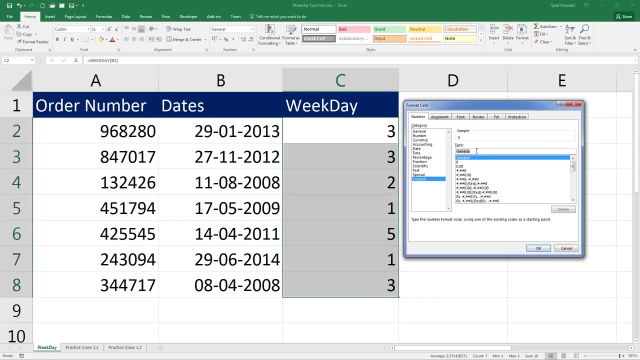 These numbers are not really going to help me. How do I know exactly the name of the day? instead of having the number, I can simply press control 1 on my keyboard to bring the format cells window on my screen, and here I select custom and in the type I will type in. 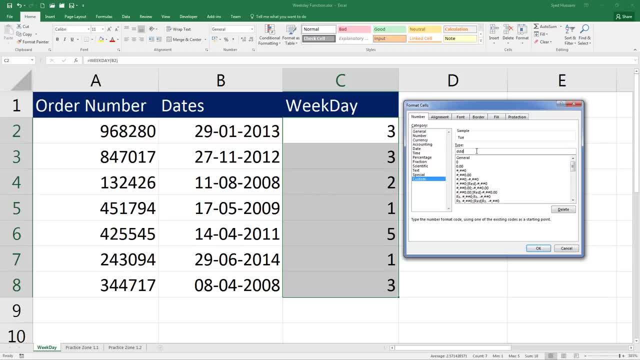 d, d, d, d is for day. if you recall from your past learning, we have done this earlier. if I type in 3 D's, it will give me a short form of the day you can see in the sample. but if I type in another day, it will give me the full name of the. 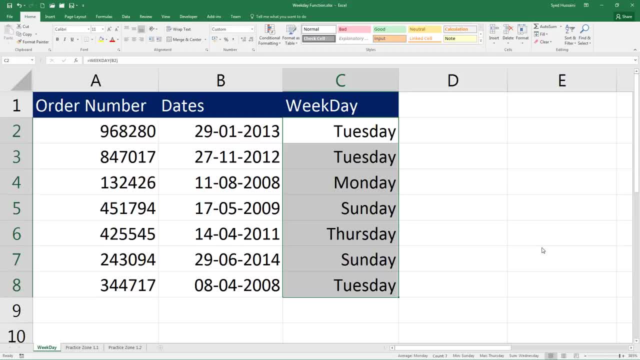 day. see that that's how we generate the weekday using the weekday function. these days listed here are visibly text, but actually they are numbers confused. let me show you how there are two functions in Excel to find out whether the given value is a text or not. so let me see if I just go ahead. type in is text and 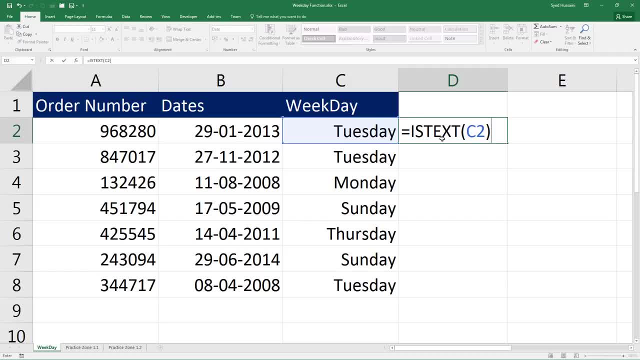 select this value. close the bracket. the moment I press enter, this function will return me the false or true. looking at the cell value, I can simply say it has to be true. but look what happens. I press enter, it says it is false. it is not a text. now let me try. is it a number? is number? let me see whether it is a number.